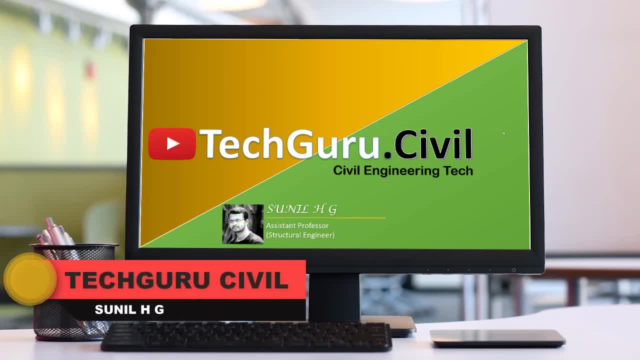 Hello friends, welcome to techurocivil, a channel dedicated to the civil engineering technology. If you like our videos, give a like and share among with your friends, And don't forget to subscribe. click on the bell icon to receive all the notification. 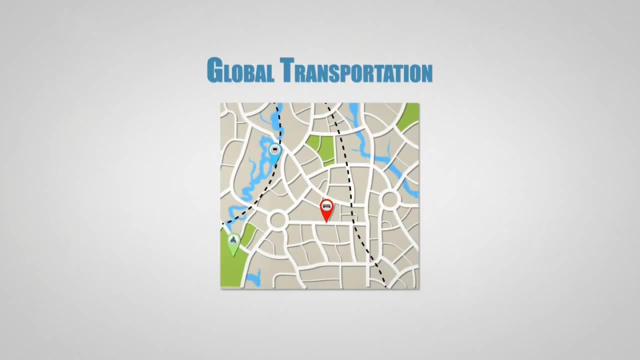 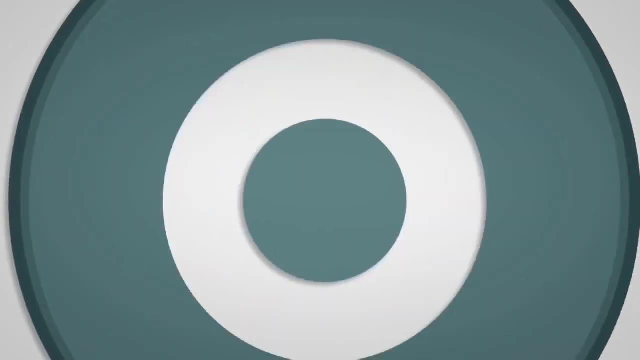 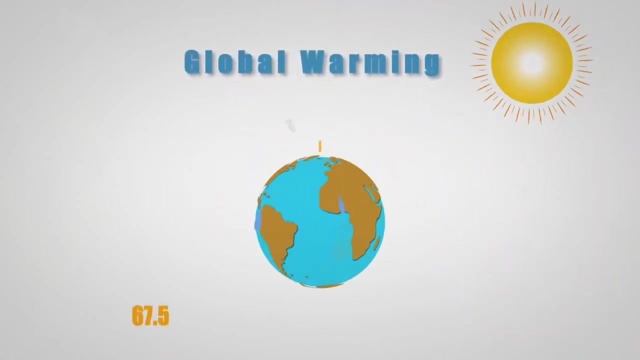 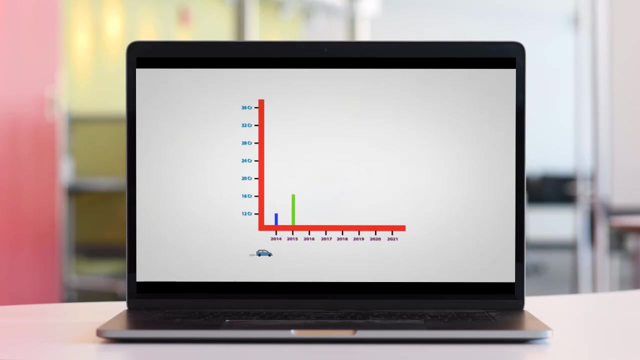 Have you ever imagined the global transportation system 10 years from now? Full of congestion, accidents, pollution leading to slowdown of economical growth, health concerns, global warming at its peak and disturbed family and social life? In 2021, the Indian roads will be crowded by three times the vehicles. 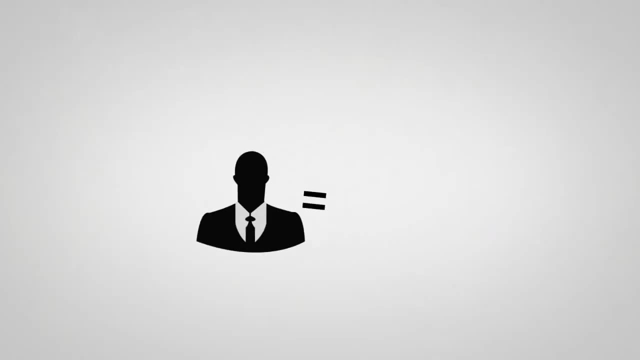 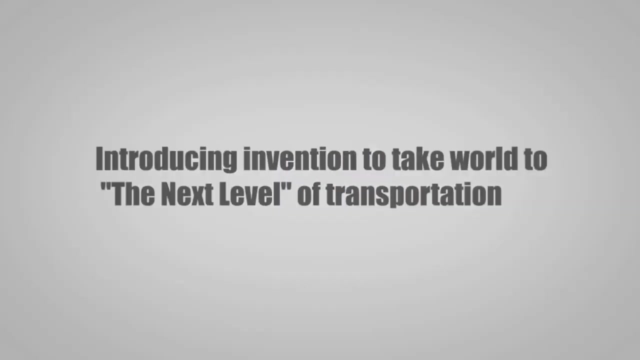 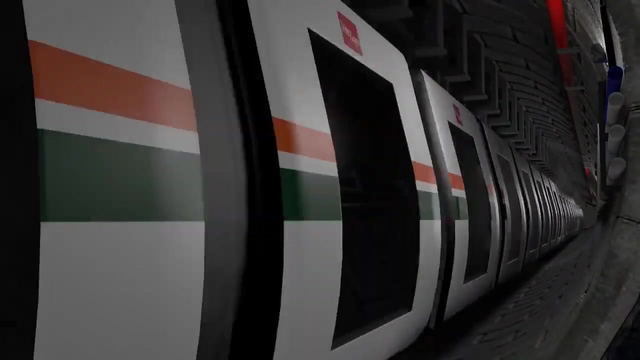 Can mankind survive this situation? The answer Is a big no. Can this situation be handled and changed? The answer is a big yes, Introducing an invention to take the world to the next level of transportation. Trans is an underground mass transportation system which runs a few feet below the existing roads. 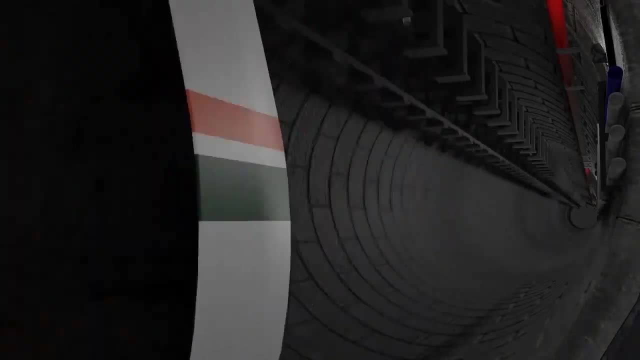 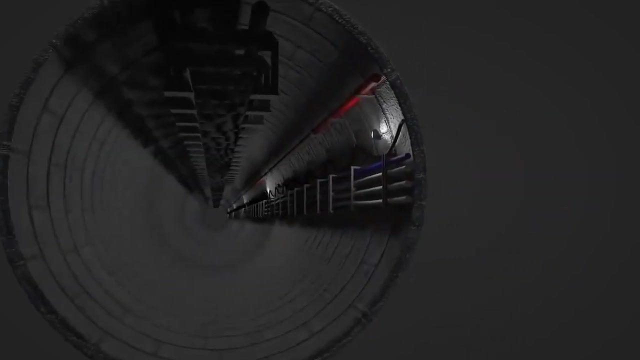 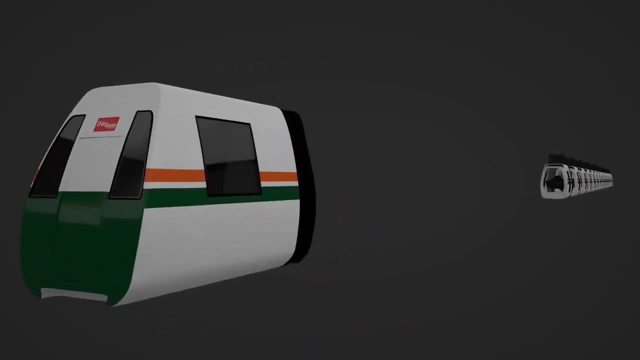 inside a swamp tunnel like a big water supply pipe with a diameter of 7 feet in circular track. Tunnels are equipped with fresh air supply and firefighting. line Trans is a collection of bogies where each bogie accommodates a single person. 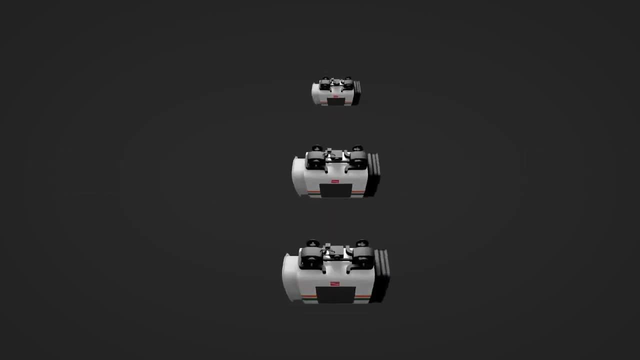 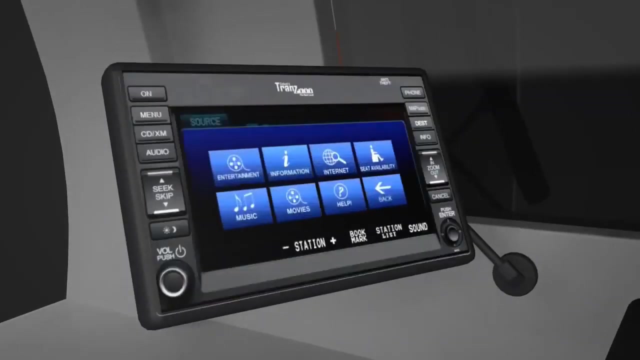 The number of bogies could be different in size depending on the need of the route and density, like 50, 100 or 200.. The bogie comes with split doors to give easy access to the traveler. Infotainment provides entertainment, information, Internet and many more facilities for a smooth and worry-free journey. 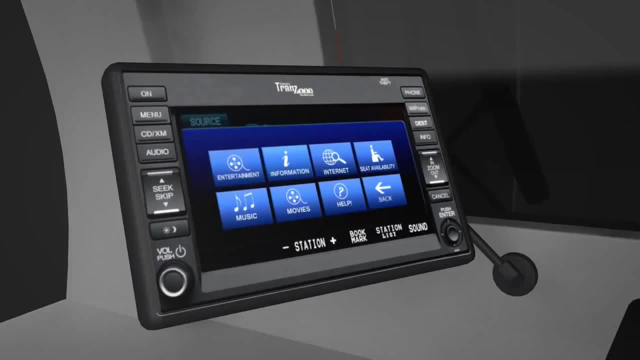 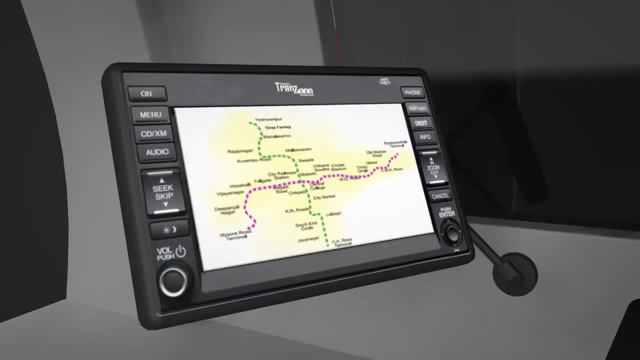 • So, if you plan to travel as a tourist or travel as a public transport during transition from country to country. • The infotainment also provides destination selection facility, which transmits available seats information to coming stations and keeps specific number of passengers ready to board the Trans. 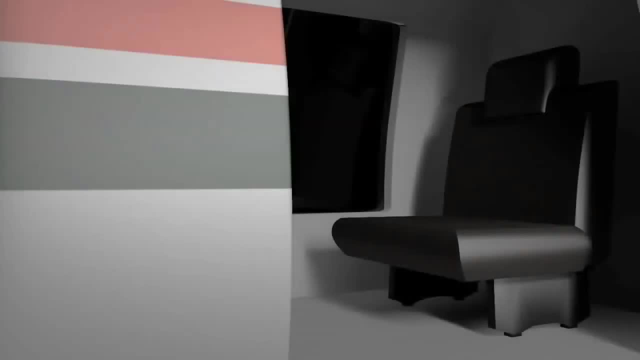 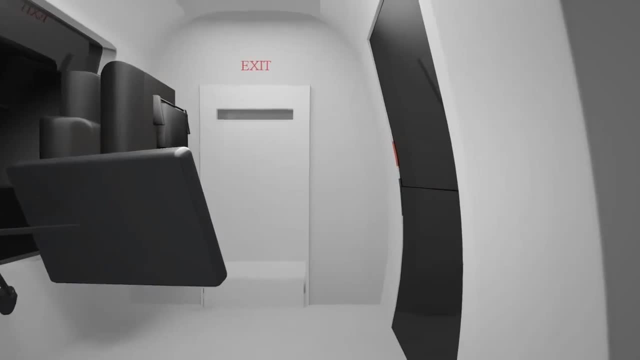 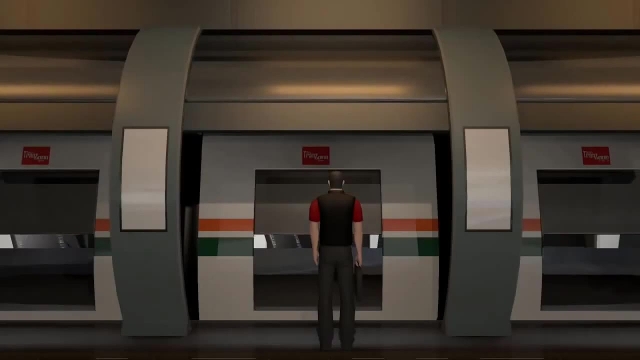 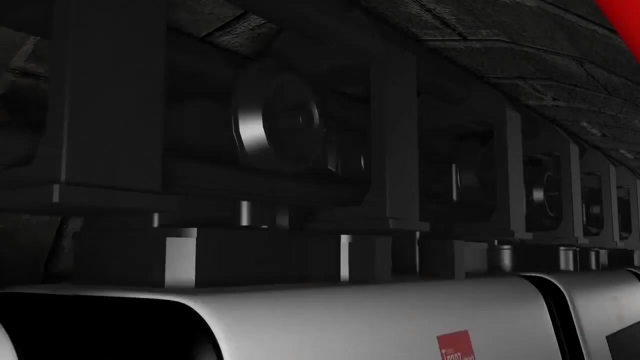 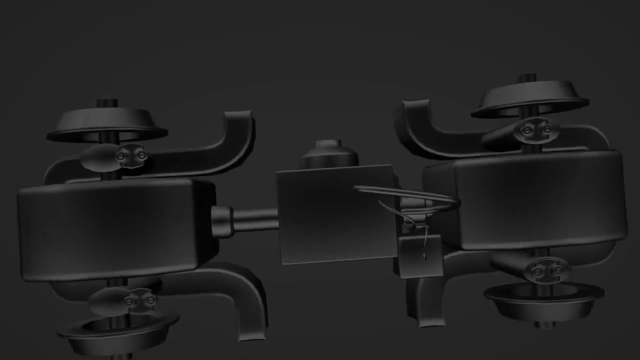 Trans during emergency via front or rear of Trans Safety doors provide safe platforms to travellers and opens on Trans arrival only Trans runs on an overhead track which makes it safe from derailing, provides a jug free journey and high speed. Trans is powered by multiple electric engines. 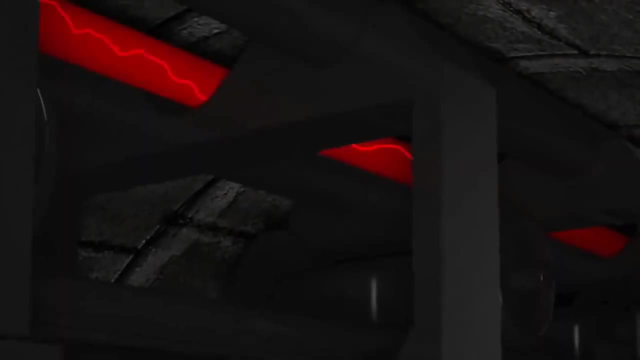 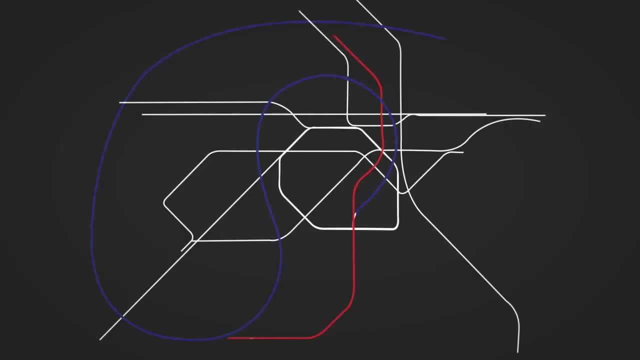 installed on the top of random bogies. Electric supply is provided through the line assembled at top of the tunnel. There could be many types of Trans tracks, like point to point, run between two main points, like dense offices to residential areas, Main points and multi-point stoppage. 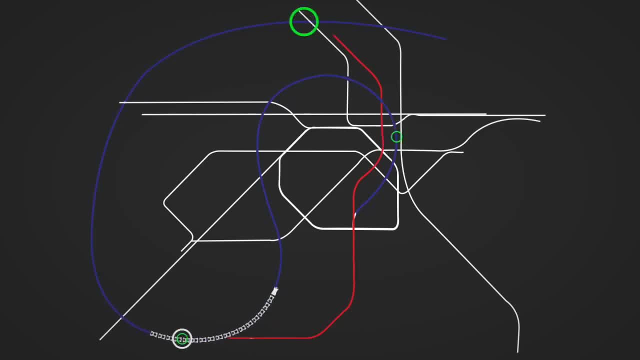 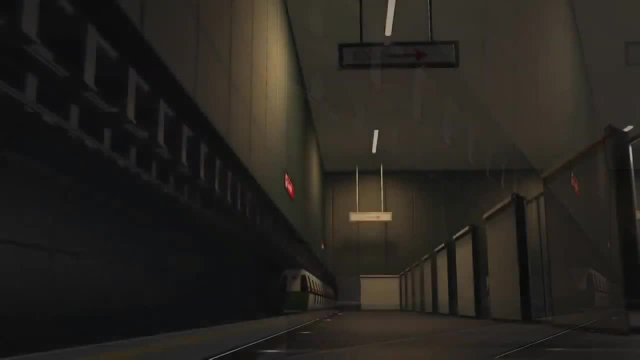 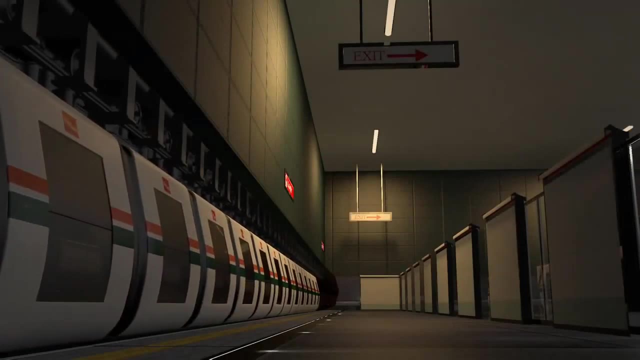 which distributes crowds equally and reduces traffic. There is also a parking or assembly area used to park Trans to reduce frequency during off hours also gives access to Trans staff for assembling, repairing and cleaning the Trans. This area can also be used for emergency exits if needed. 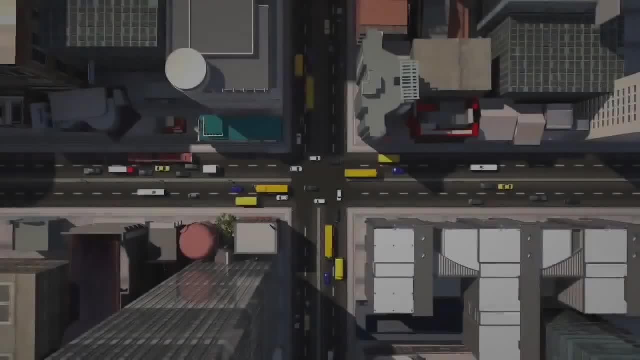 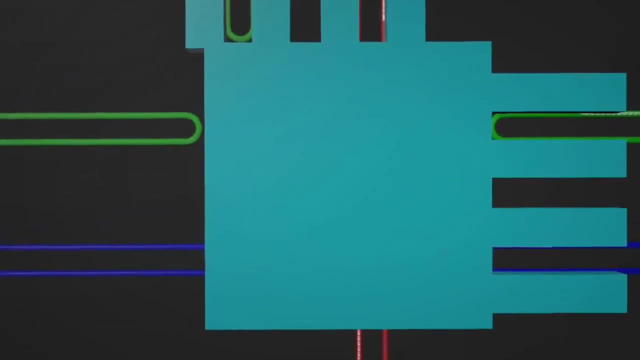 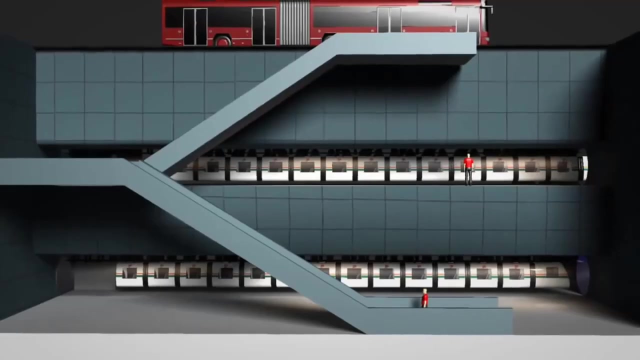 The main stations are below any square of the city where two or more tracks intersect these stations, giving access to more people and even more people. The main station is located between two or more people and easy transfer facilities. Sub stations are stoppages where main points and all points Trans stops. 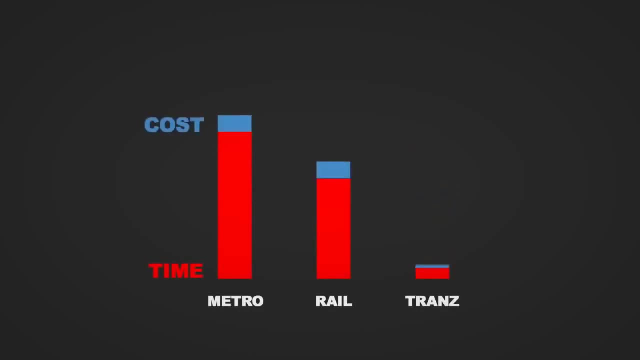 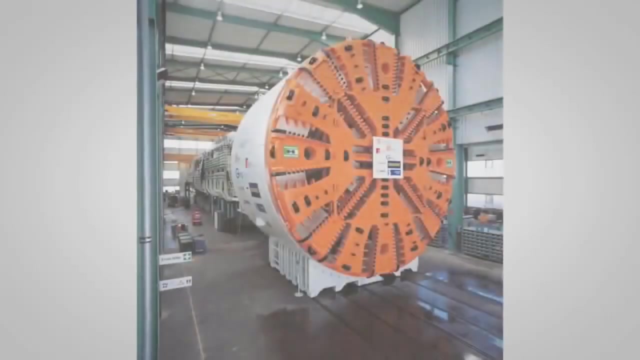 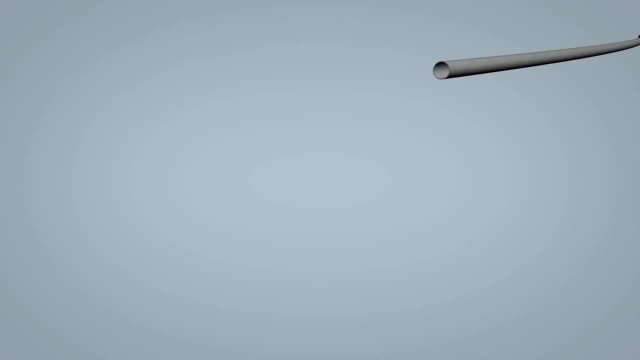 Trans can be constructed in 90% less time and cost comparing to other mass transit systems like the metro and rail. A small tunnel boring machine provides faster construction and it also does not interrupt ongoing traffic. As per our study, each TBM can construct more than one kilometre of Trans track each day. 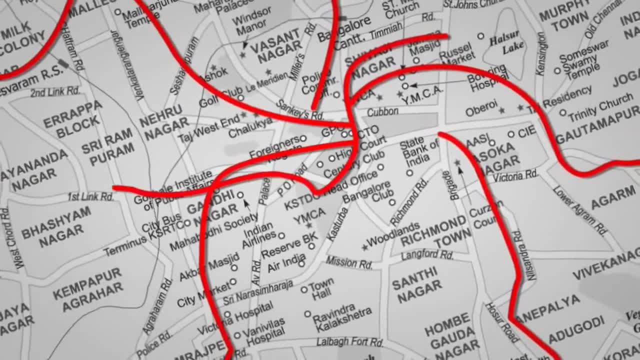 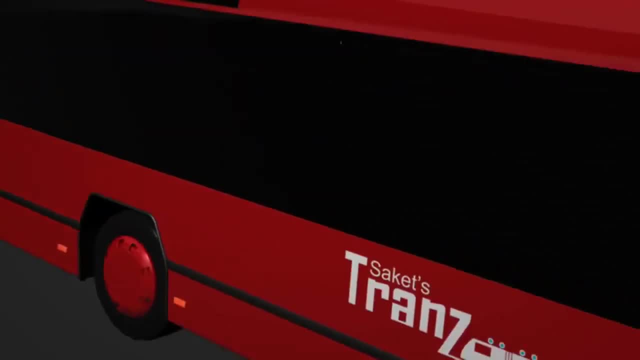 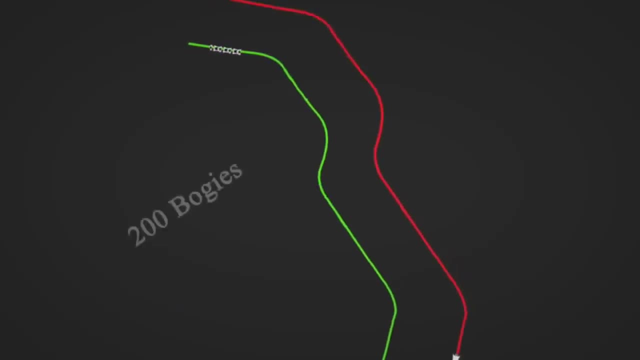 and with the help of 50 TBMs, within six months the whole city of Bengaluru can be constructed and become functional. Feeder service will provide accessibility to Trans from all parts of the city. Each Trans track with 200 bogies transport 12,000 passengers every hour. Eachkah between two points each way.